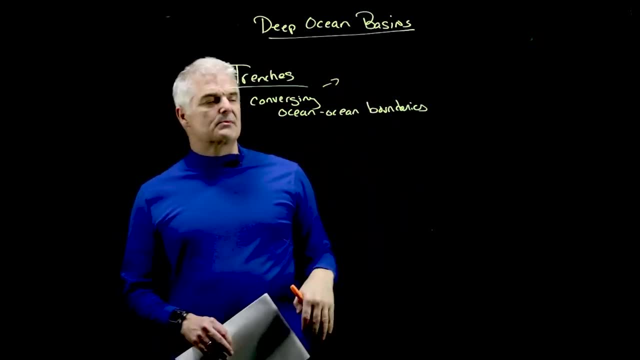 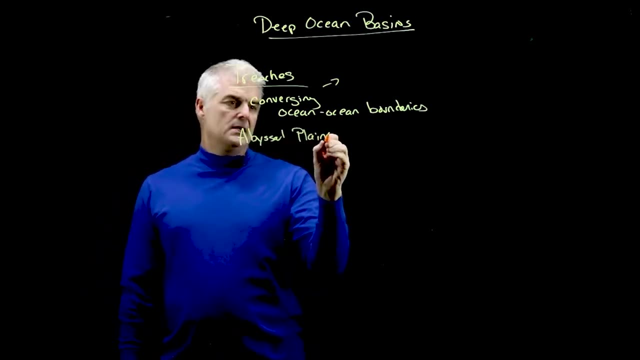 what's causing this? The cause is that you've got the denser plate subducting underneath the lower plate. Make sure you write that down in your notes. The second sort of feature we see is this is the abyssal plains. This is the flat part of the under. yeah, it's flat, So for vast regions. 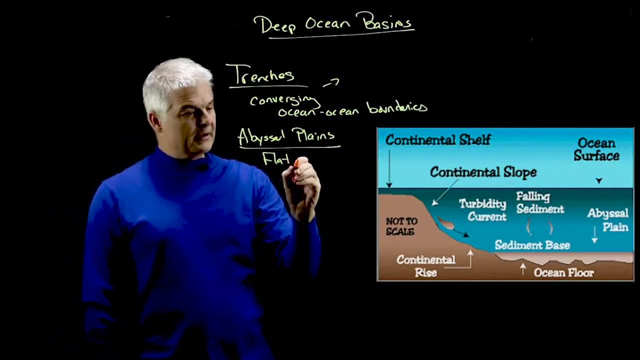 of the ocean. it's just flat Now. it's flat, but it's not flat. It's flat, but it's flat. It's flat, but it does have sediments on top of it- Sandy dirt. Now we've got a whole section on sediments. 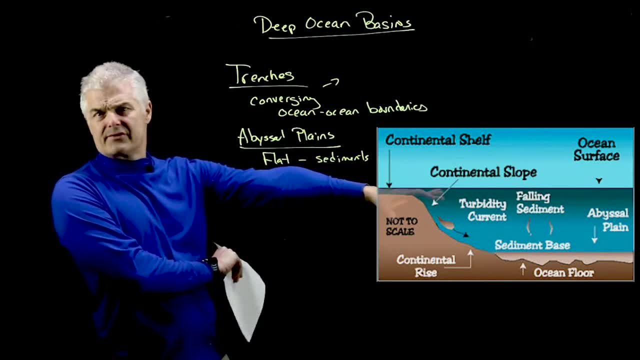 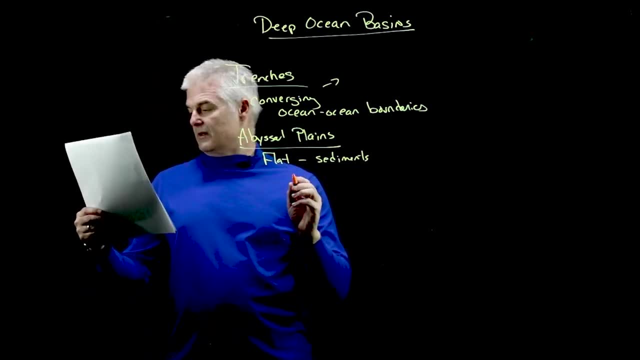 coming up later, So we'll get there later. but it's just the flat parts of the ocean, So lots of those exist. By the way they're found, the abyssal plains are- I should make a note here. 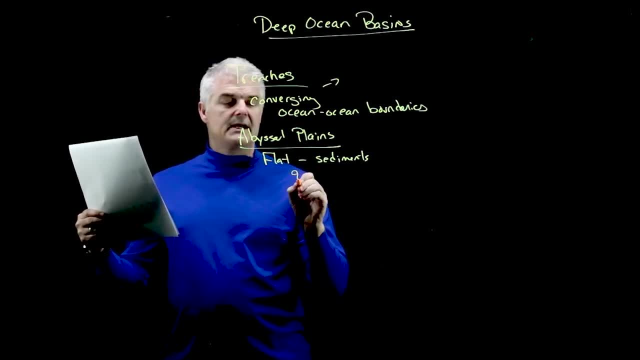 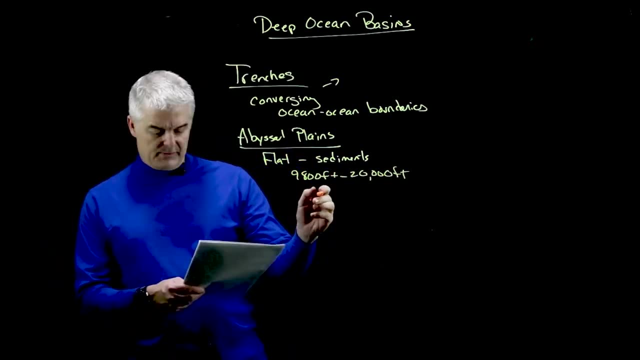 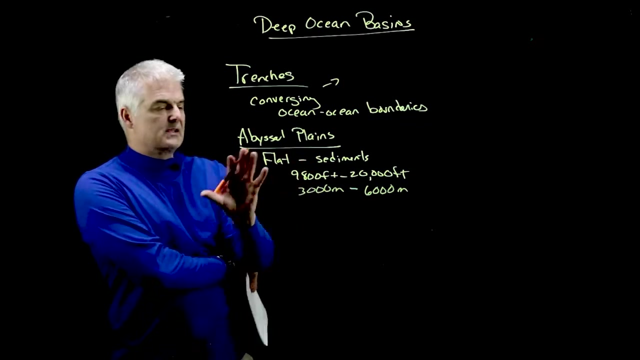 they're underwater. They're found at depths between 9,800 feet to 20,000 feet. They're flat, but they're going to be at different feet. By the way, in kilometers that's 3,000.. It's 3,000 to 6,000 meters. So we've got these flat parts and they can have anywhere between so they're deep 10,000 feet down right. 3,000 meters is kind of the minimum, and then they can be even deeper. So these are the deep parts of the earth And the question is, you might ask, 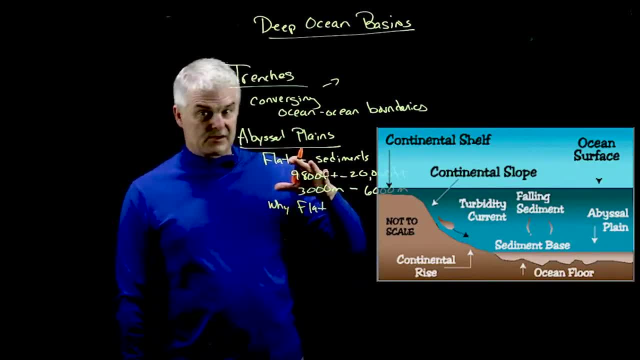 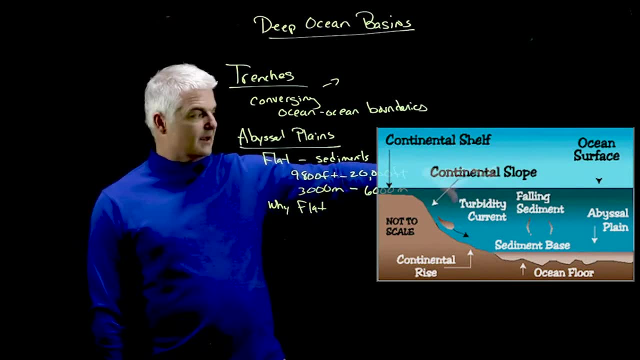 is: why are these so flat? The reason they're flat is because, over time, the sediments that have come from the continents, right from rivers and mass wasting, all that stuff that we've talked about- they're spreading out. There's all kinds of currents in the ocean. that's moving things. 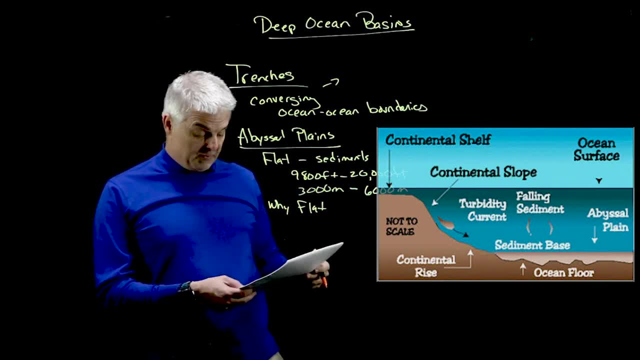 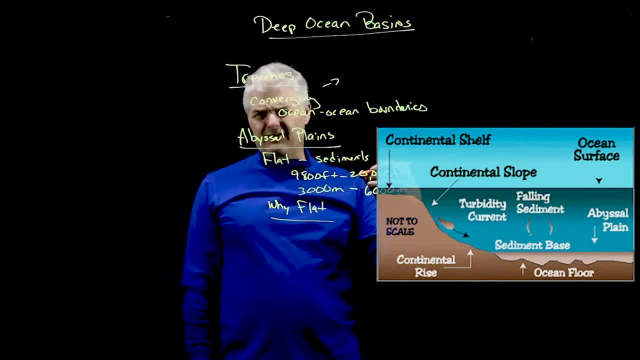 around And then over time- it could be centuries- they settle. In fact, speaking of how long that they do that, I have it. I guess it comes up in a later video. It talks about how long it takes, something like 50,000 years for certain, like centimeters, But over years that sediment. 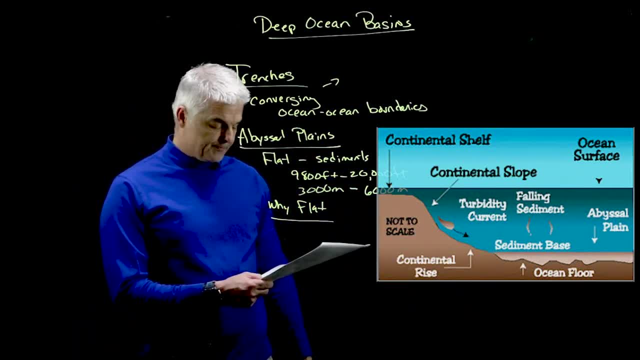 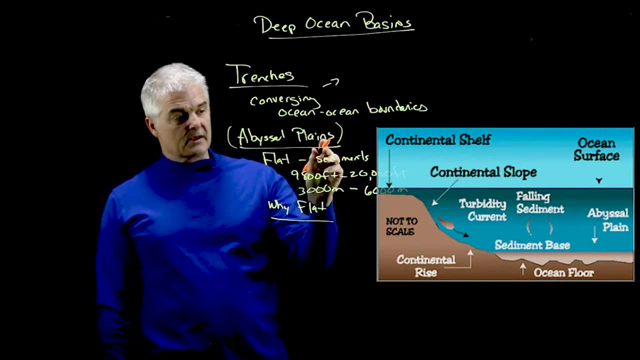 settles to the bottom of the ocean And it turns out, if you look around the oceans, that the Atlantic has the most abyssal plains. And then you might say: because what's causing this is the buildup of sediment And the Atlantic Ocean. 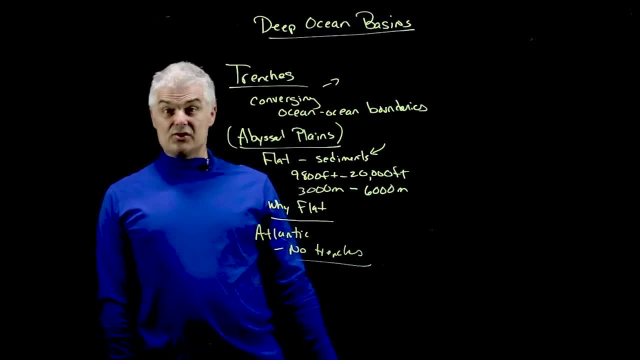 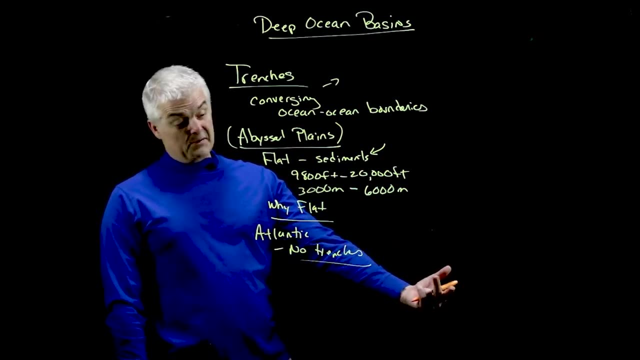 doesn't have any trenches. There's no converging plate-plate boundaries, because what happens with the trench? if you think about it, it's like the hole that can collect more sediments And there's no place for that. So you get the flat regions in the Atlantic Ocean because it doesn't have. 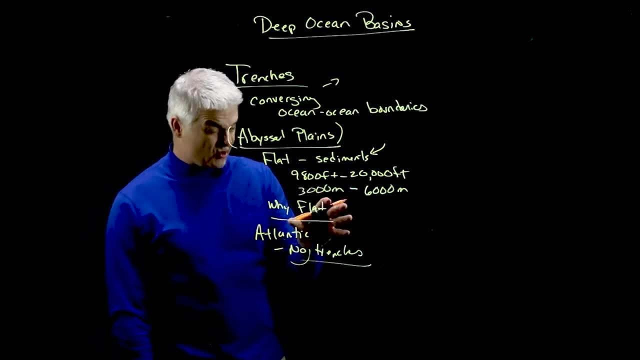 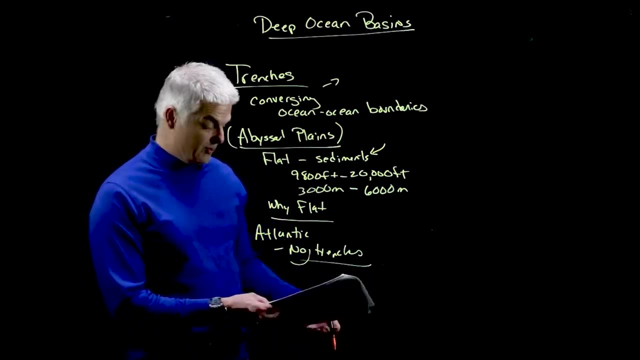 probably- no is an overstatement- but very few trenches, And without the trenches you're not going to get a place to collect the sediment, So that's why you find the most abyssal plains in the Atlantic Ocean. The next one is a seamount- Kind of a cool term, Essentially what this is, of course, 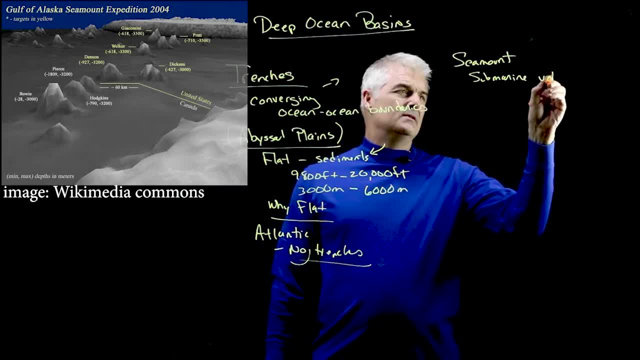 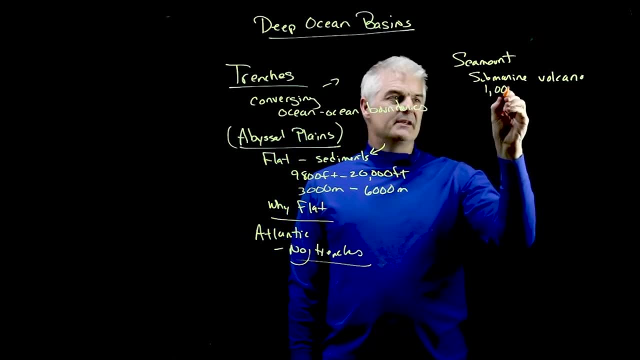 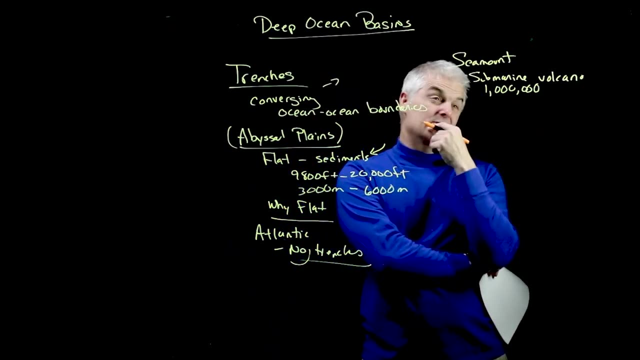 is. this is a submarine volcano, Now underwater volcano. You know how many underwater volcanoes there are? A million, A million, A million, Yeah, A million underwater volcanoes. I think it's pretty awesome, And these are all over the planet. You can find all these little submarine. 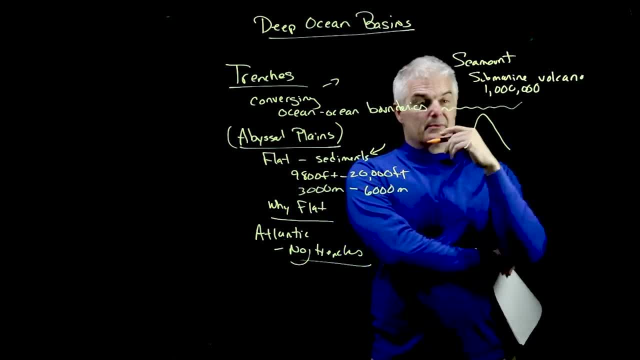 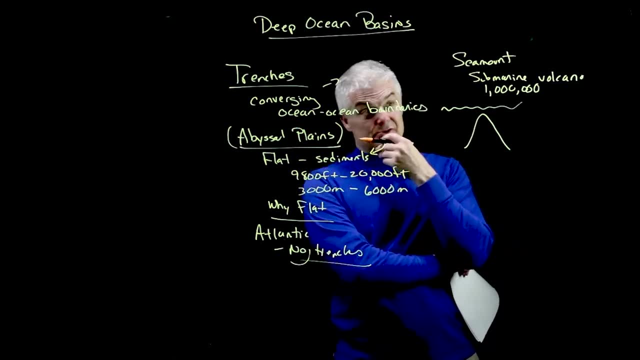 volcanoes, And so they rise up, but they never make it. Well, they don't always. They don't always make it up to the surface, And so underneath the ocean you can find a seamount. I think seamounts are pretty cool. Some seamounts do make it to the surface of the Earth And, of course, one example would be the Hawaiian Islands- Ooh, you've been to Hawaii on the beach, Get that tan right. Also, the Aleutian Islands and the Azores. You can find seamounts, lots of places, And most of these, some of the ones I've just listed, are ones that do come off to the surface of the Earth. 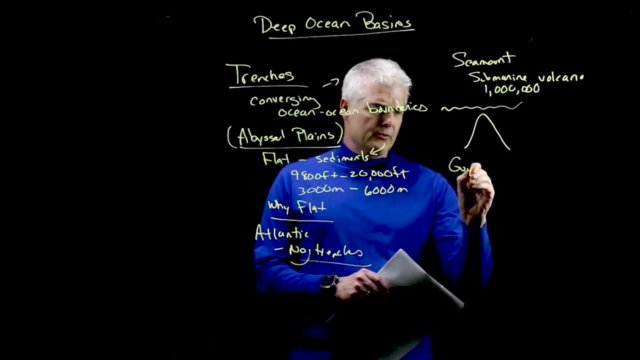 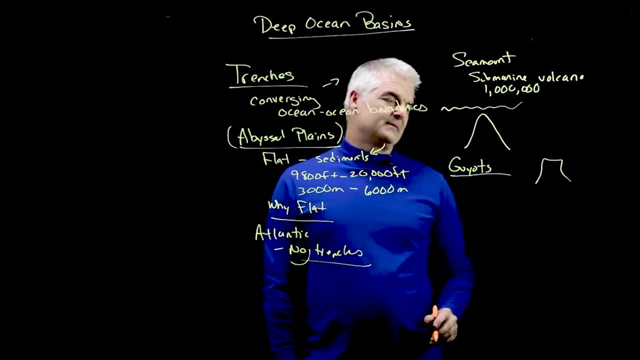 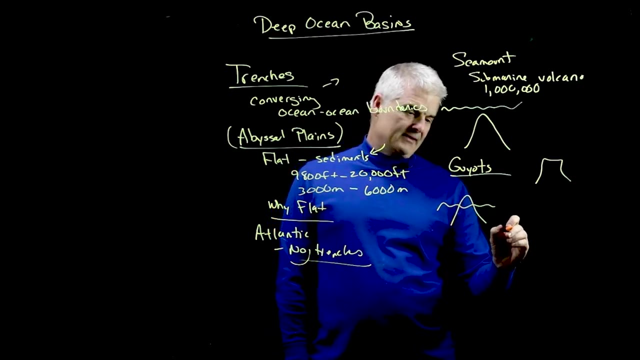 The next one's called a guy-out- Guy-out Like a side-out in volleyball, Or guy-outs. A guy-out looks like this. You know what it is. It's a seamount that made it to the surface And then the wave action flattened this. There you go, And now it's a flat top, And sometimes they'll even 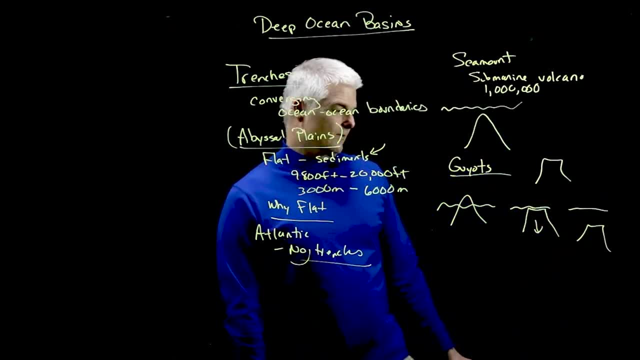 sink a little bit more And he's even sunk further and further. So at one point he was a guy-out of the ground and of the water, pardon me, and then he sunk. So this is a guy-out We. 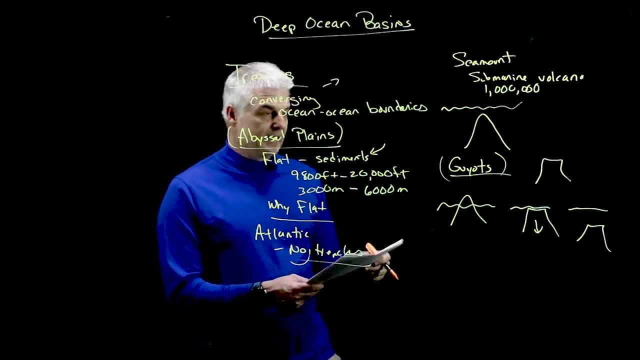 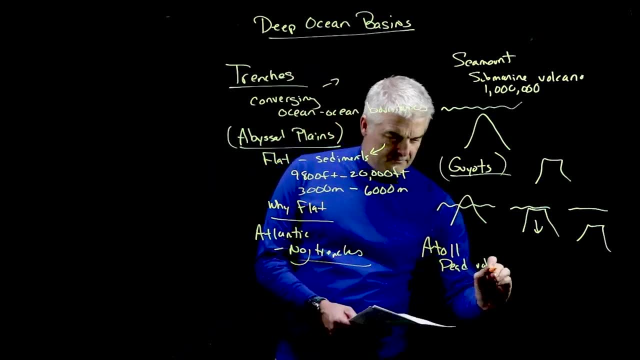 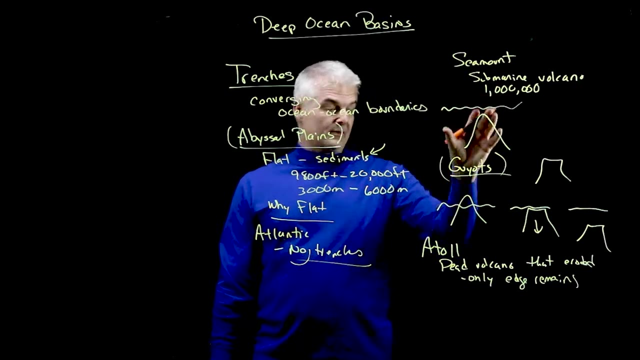 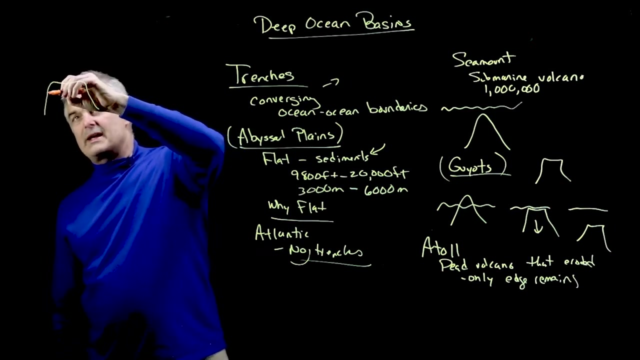 sign these all over the place, And then I think the coolest one maybe is the atoll. Now, this is a dead volcano that eroded and only the edge remains. It's actually a function of the guy-out. The guy-out's an underwater volcano, And so what happens is you get the guy-out here, But 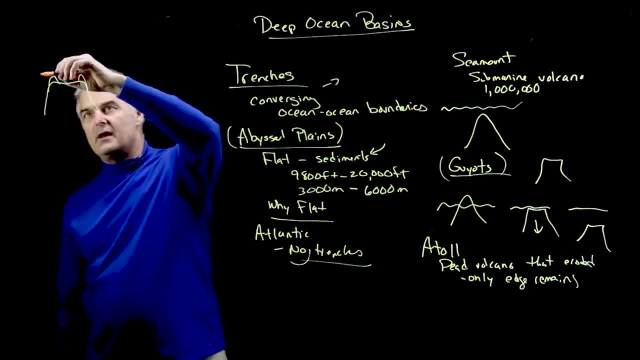 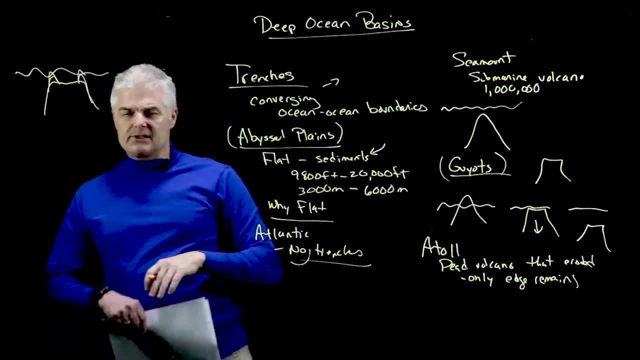 the volcano that has a caldera. This looks like a weird cat, And what's happened is you've got a little bit of the land. Well, let's take a look. Take a look at this atoll And it's just a ring. 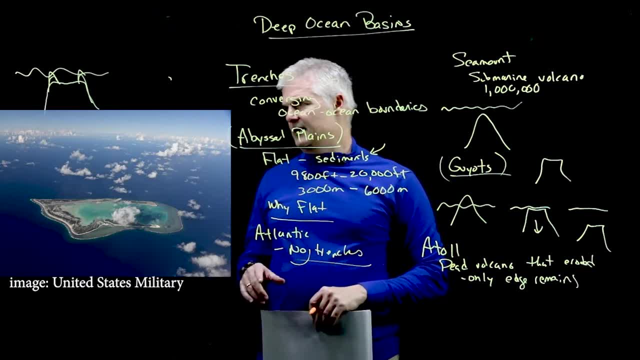 It's a ring of a little bit of land, if you can kind of see that, And it's risen up because it's again one of these guys over here. And then the thing that's really cool about atolls at least. 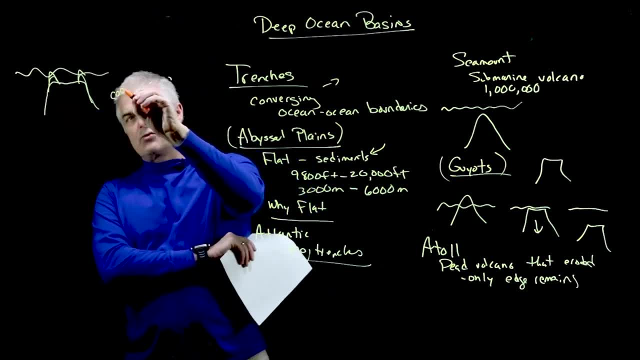 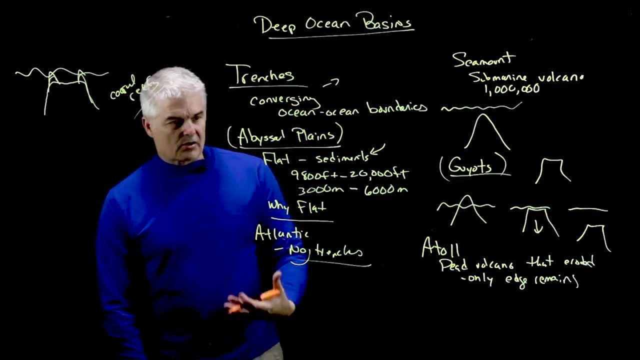 in warm water is that this is one of the biggest places where we see coral reefs And the diversity of life that you see in a coral reef. maybe you had a chance to go snorkeling- maybe in Hawaii or some other place like that- and you've seen the coral reefs and the beauty and the majesty And 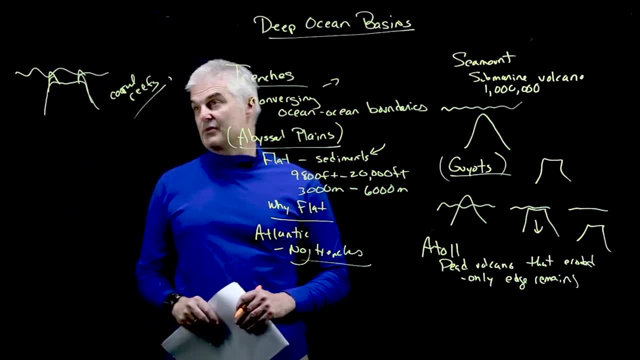 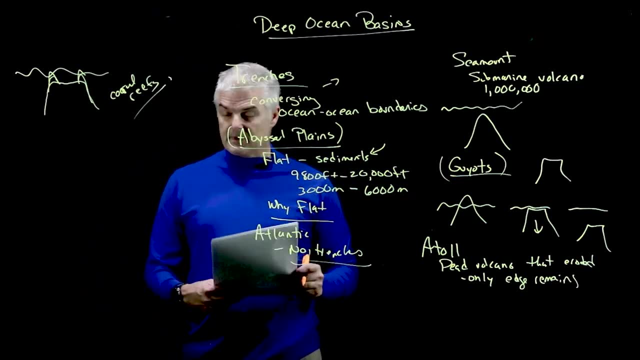 when we see all the colorful fish. coral reefs is one of the most amazing places, And there's a lot of concern because maybe the coral reefs are dying around the world. It's quite a sad thing. And then the last one we want to talk about. 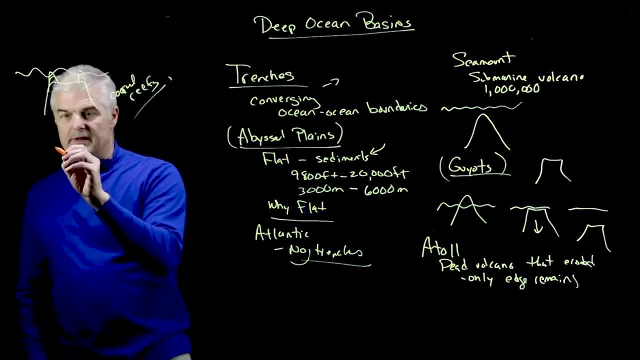 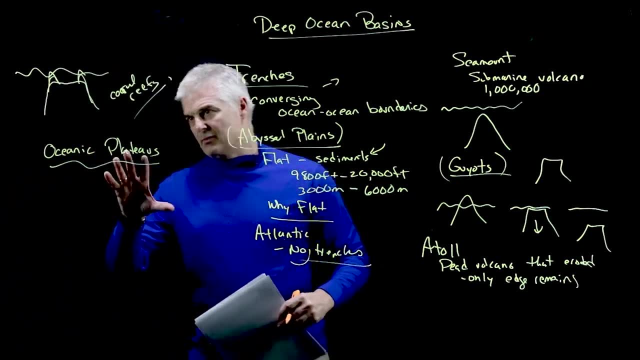 I think it is yeah. And then the last one we want to talk about I think are pretty awesome too- is the oceanic plateaus. So it turns out that when we look at different parts- take a look at this map right here- is that in this map you can see some different regions. 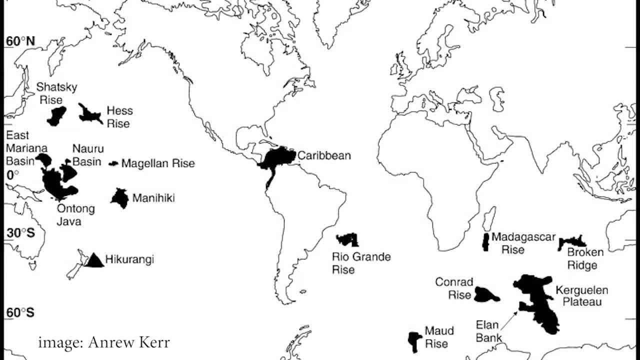 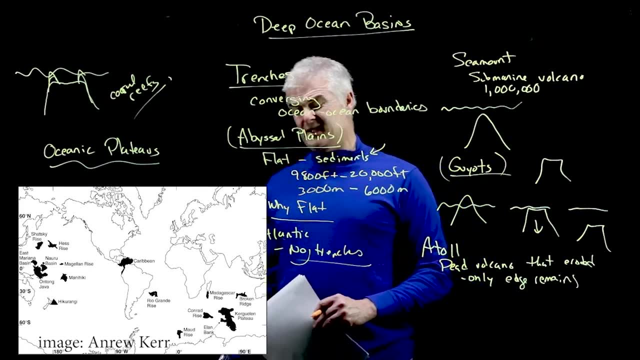 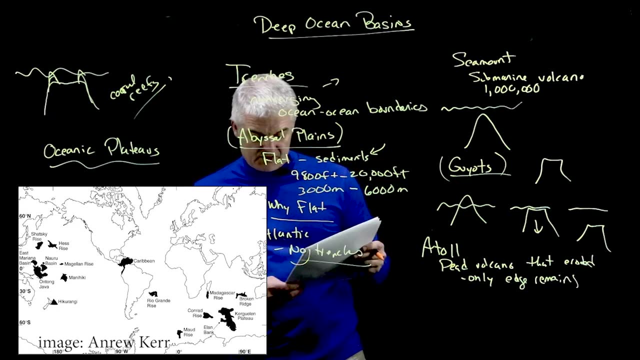 around the earth that are plateaus. So basically, these are rises, large rises underneath the ocean that are much, much less shallow, And it turns out that some of these were actually continents back in the day that have eroded away. I think one of the cool ones is this one called 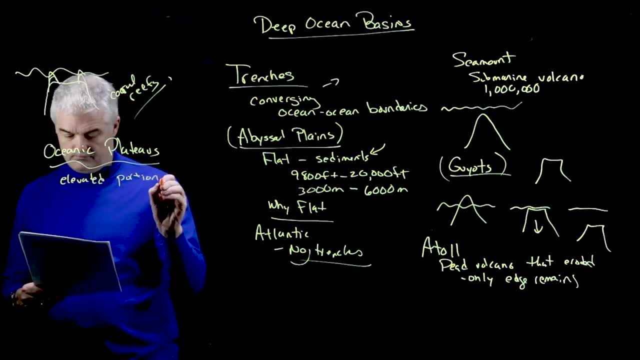 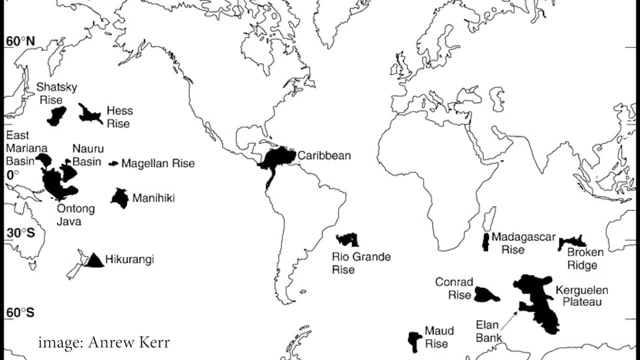 actually, let's just define this. first, An elevated portion of the seafloor is flat, Fair enough. Now, one that's fascinating to me, if we look down here, is a place called the Kreligin Plateau. It's off the coast of Antarctica. 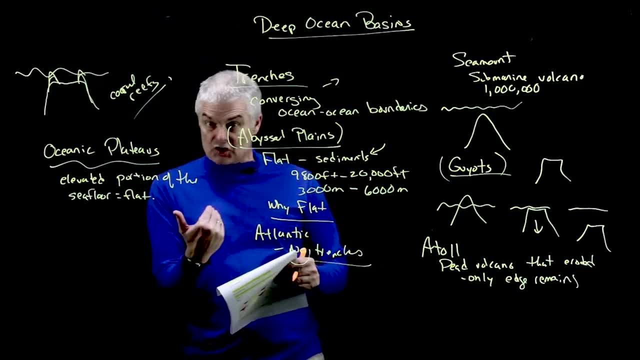 It used to be connected to India and Australia And it broke away and it sunk And if you go down there, you find fossils of animals- animals who lived on the Earth- Terrestrial, not aquatic, And down there we have- it's a sunken continent. 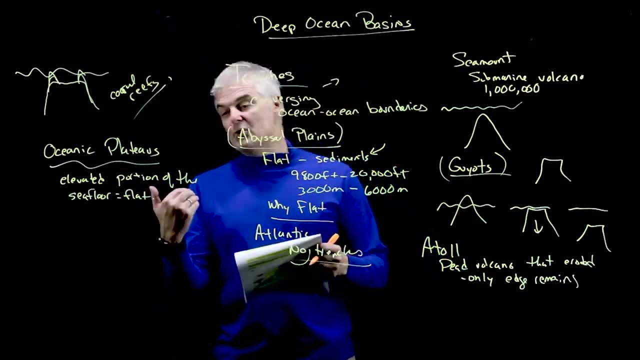 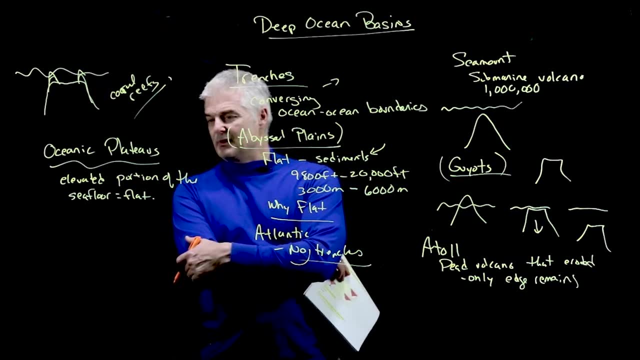 Is this the lost continent of Atlantis? Probably not, Because this is one of the remotest places on the planet- Antarctica, It's cold, All this kind of stuff. It is an amazingly weird place. I just got sort of entraptured.